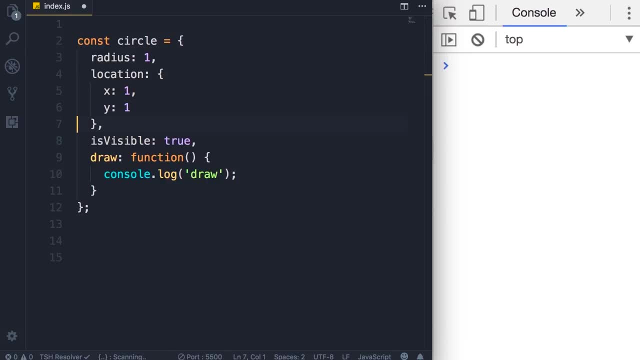 the second circle and show you how to create a factory function. So factory function just like a factory producing products, these factory functions produce objects. So we define a function and call it create, discover. Now we're going to move this definition of the circle object inside of our factory function. 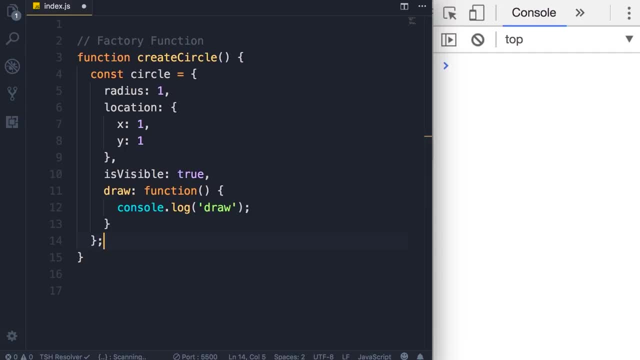 So we have a circle object here. Finally, we need to return this. Now, one way is to return it like this: But we don't really need this circle constant defined because we're not going to reference it anywhere. we only want to return it so we can make this code shorter. 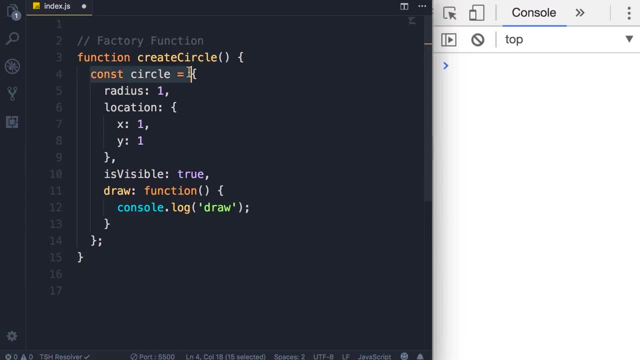 by removing the circle constant and simply returning this object. so whenever we call the create circle function, we'll get a circle object. however, we have hard coded these values here, so every circle that is created by this function, its radius will be one. that's not what we want. maybe we want to have a circle with a bigger radius, so we want to pass radius as a. 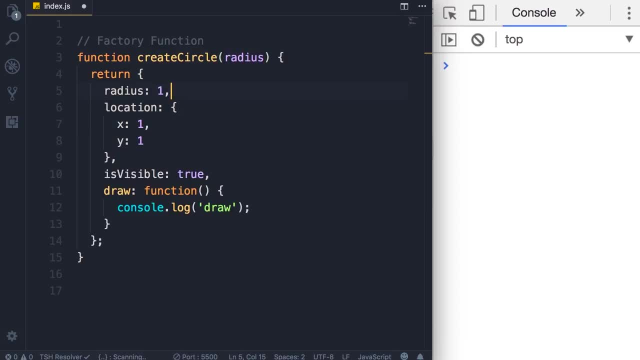 parameter here, so radius, and then instead of hard coding one, we want to set the value to this radius argument that we supply when calling this function. similarly, we can add another parameter here, like location, and instead of hard coding this object here, we can simply set location to this location argument. however, 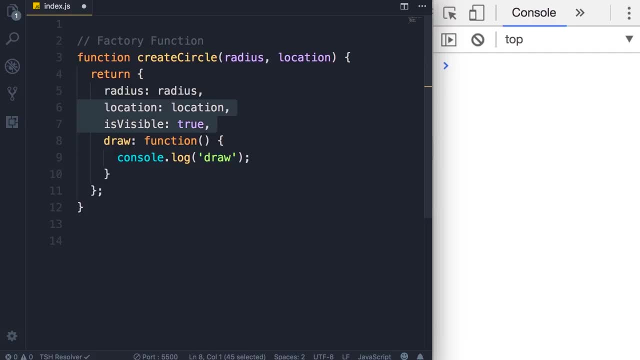 you can see that we have a circle with a bigger radius, so we want to pass radius as a parameter. for simplicity, i'm going to remove these two properties. location and is visible so we can focus on the core of factory functions. so let's delete these properties. we don't need the location. 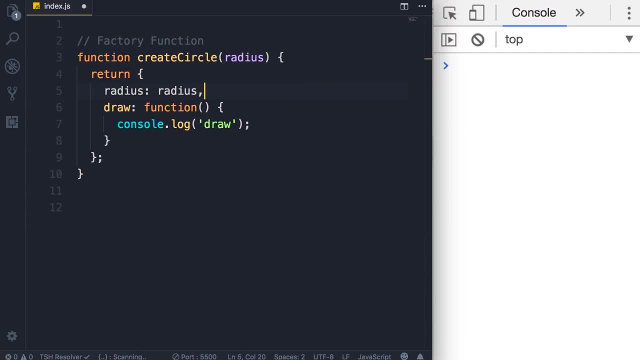 parameter either. now we can make this code a little bit shorter. so in modern javascript, if our key and value are the same, we can make our code shorter by removing the value and simply adding the key. so that is exactly equivalent to this code. right, so that is better. next we have our draw method. there is also a shorter syntax. 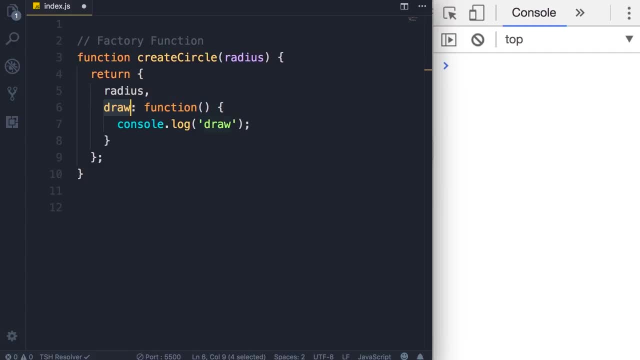 so define this method. so, instead of defining it as a key value pair, we can define it like this: so draw parenthesis and code block. this is similar to how we define a function outside of an object, right? so if you want to define a function, this is how we define it, right? so we have the function. 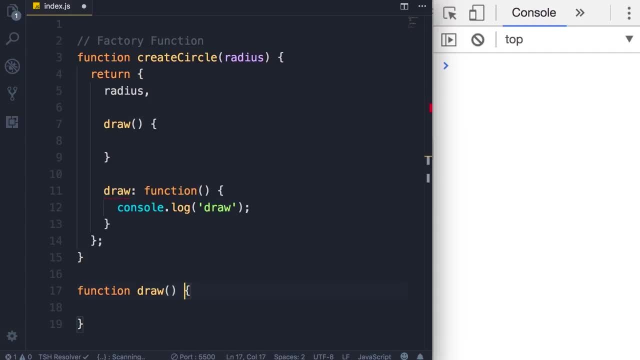 keyword and we have the function keyword and we have the function keyword and we have the function means. and then the name of the function, parenthesis and code block. now, when we put this inside of an. then the name of the function, parentheses and code block. now, when we put this inside of an. 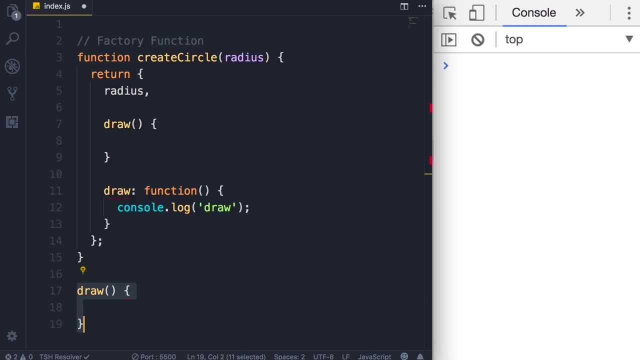 object. basically, we are dropping the function keyword and simply adding this inside of the object. you can see, this syntax is a little bit shorter than what we have here, so let we have here. so let me delete this and move this consolelog statement in our draw methods. so so now we have a factory function we can 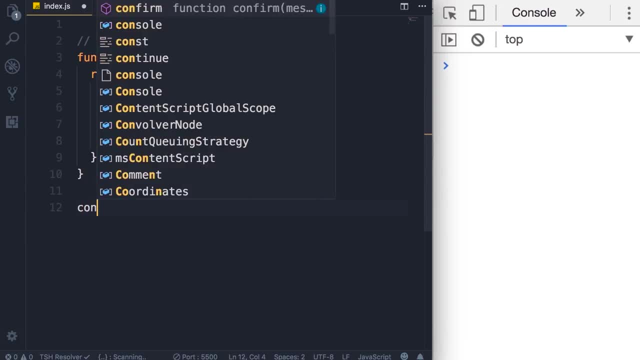 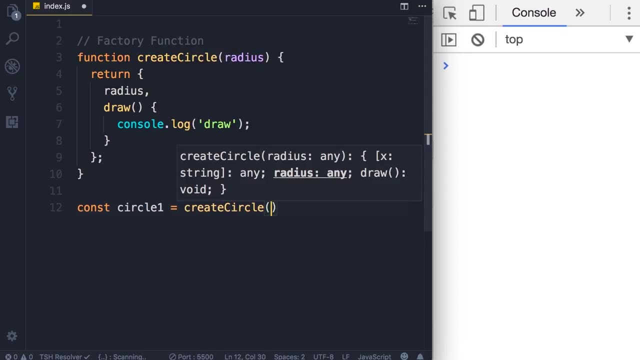 can simply call this to create a circle object. so I'm going to define this constant circle 1 and call the create circle function and pass 1 as the radius. now let's log this circle object on the console, circle 1. save the changes so you can see radius is set to 1. we also have this draw. 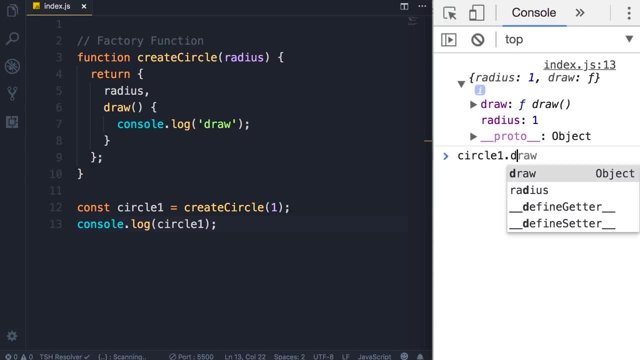 method. so we can call circle 1, draw. and here's our draw message on the console. now the beauty of this factory function is that we have defined our logic in one place. so we can call this function with different values or different arguments. we get different circle objects, but we have defined 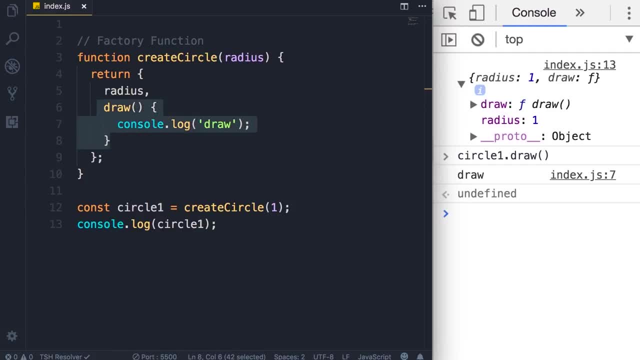 the draw method only in one place. so if there is a bug in this method that we need to fix in the future, there is a single place that we need to modify. so now I'm gonna create another circle: object circle. to create circle, I'm gonna pass 2 as the radius. let's log this on the console circle to save the changes. look we.